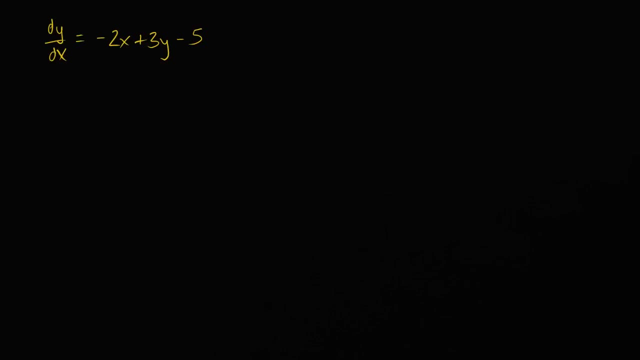 So let's get a little bit more comfort in our understanding of what a differential equation even is. And so here we have a differential equation and we haven't started exploring how we find the solutions for differential equations yet, but let's just say you saw this. 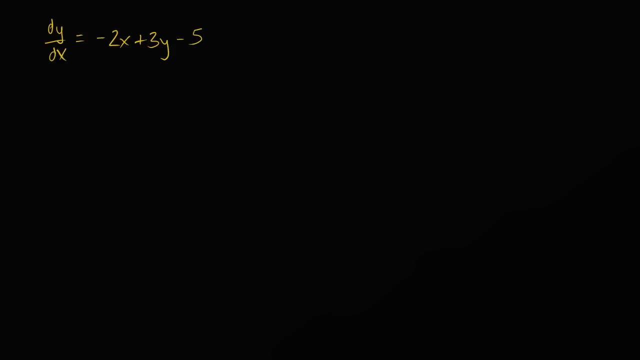 and someone just walked up to you on the street and says: hey, I will give you a clue that there's a solution to this differential equation. that is essentially a linear function where y is equal to mx plus b, and you just need to figure out the m's and the b's. 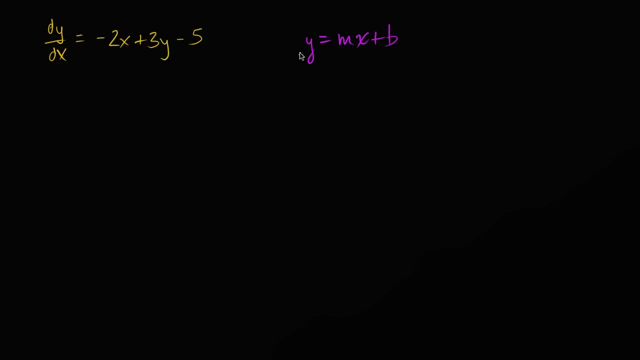 or maybe the m and the b. that makes this linear function satisfy this differential equation, And what I now encourage you to do is pause the video and see if you can do it. So I'm assuming you have paused it and had a go at it. 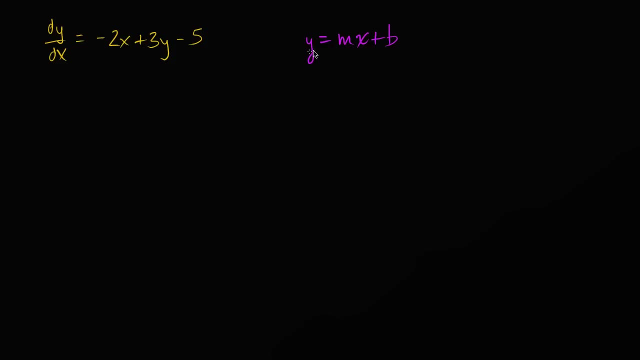 so let's think this through together. So if we know that this kind of a solution can be described in this way, we have to figure out some m's and b's here. this is telling us that if we were to take the derivative of this with respect to x, 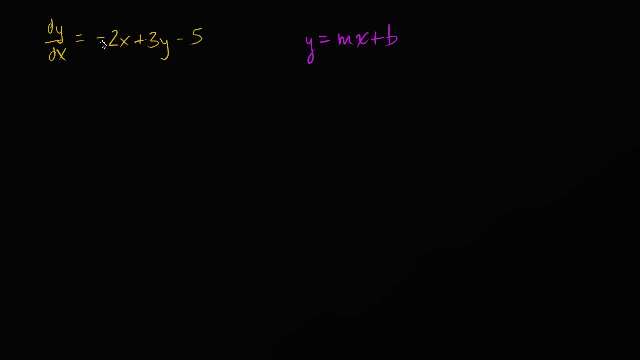 if we take the derivative of mx plus b with respect to x, that that should be equal to negative two times x plus three times y. well, we know, y is this thing minus five, and that should be true for all x's. 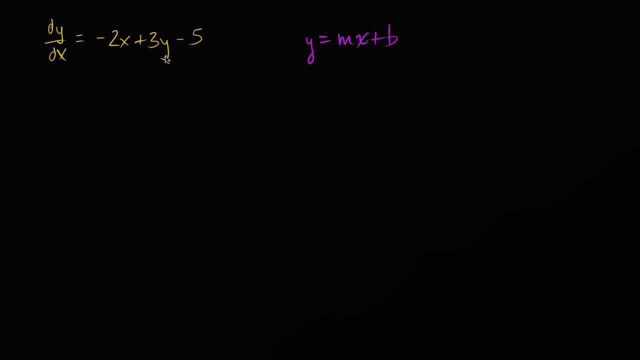 In order for this to be a solution to this differential equation. remember, a solution to a differential equation is not a value or a set of values, it is a function or a set of functions. So, in order for this to satisfy this differential equation, 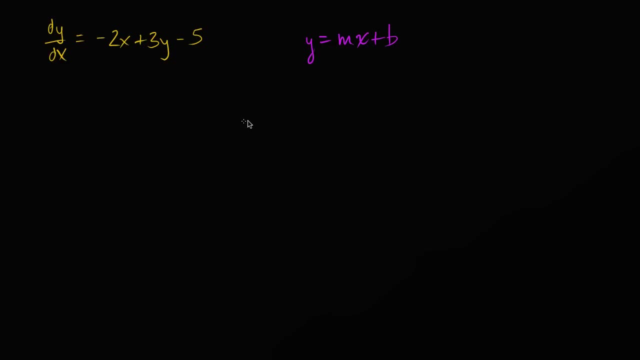 it needs to be true for all of these x's here. So let's work through it. Let's figure out first what are dy dx's. So dy dx- we'll just take the derivative here with respect to x. dy dx is derivative of mx. 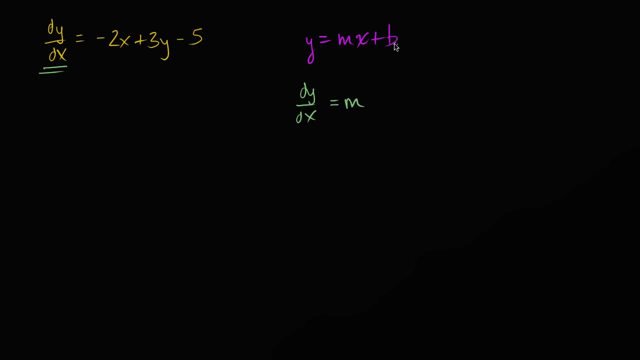 with respect to x, it's just going to be m and, of course, derivative of b with respect to x is just a constant, so it's just going to be zero. So dy dx is m, so we could write: m is equal to negative two x. 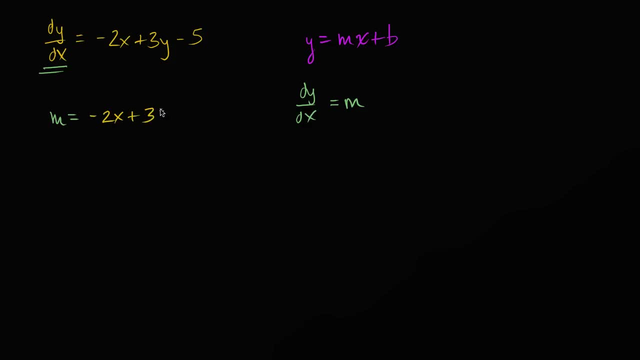 is equal to negative two x plus three times, and instead of putting y there, I could write mx plus b. So remember y is equal to mx plus b And, just as a repeated reminder, this has to be true for all x's. 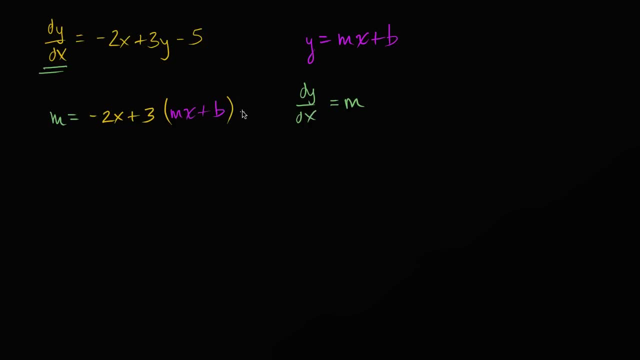 Mx plus b, and then, of course, we have the minus five, And so if you weren't able to solve it the first time, I encourage you to start from here and now figure out what m and b needs to be in order for this equation right over here. 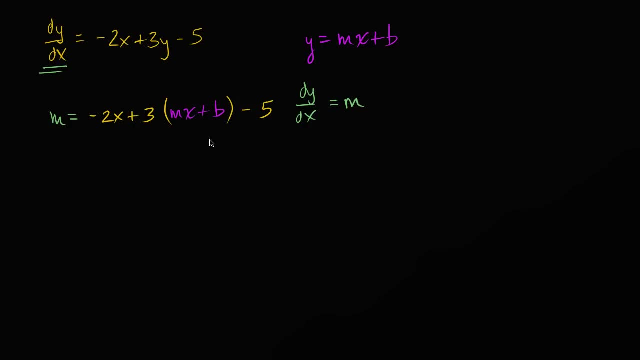 in order for this to be true for all x's, in order for this to be true for all x's. So I'm assuming you have paused again and had a go at it. so let's just keep algebraically manipulating this and I'll just switch to one color here. 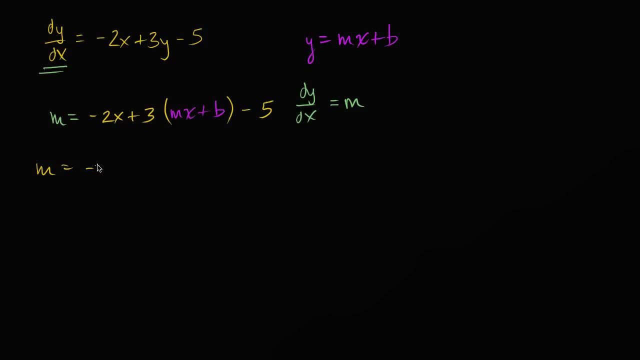 So we have m. m is equal to negative two x plus. if we distribute this three, we're going to have three mx plus three b, and then, of course, we're going to have minus five, And now we can group the x terms. 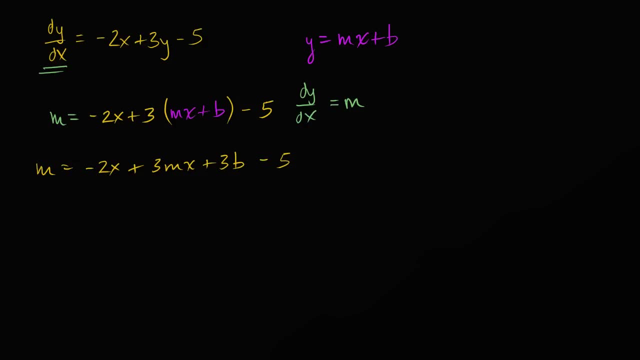 so if we were to group, if we were to group, let me find a new color here. maybe this blue. let me find a new color here. maybe this blue, let me find a new color here. let me find a new color here. 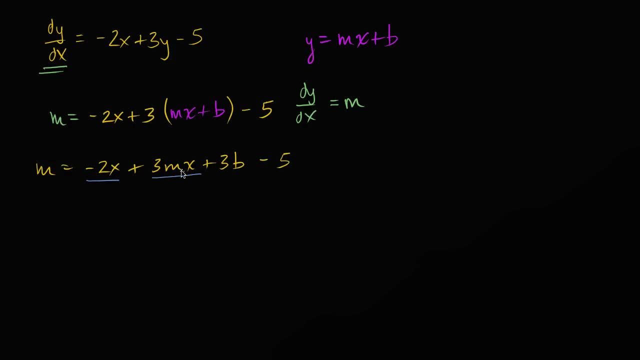 maybe this blue. So if we were to take these two and add them together, that's going to be negative two plus three m times x, or we could write this as three m minus two times x, and then you have your constant terms. 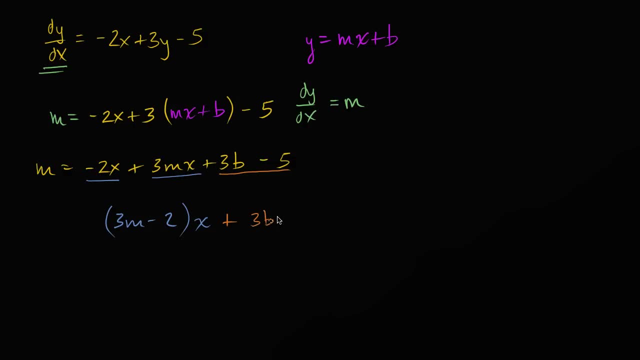 so you have these terms right over here. so plus three b, minus five, and of course, that's all going to be equal to m. That's going to be equal to m. Now, remember, this needs to be true. this needs to be true for all x's. 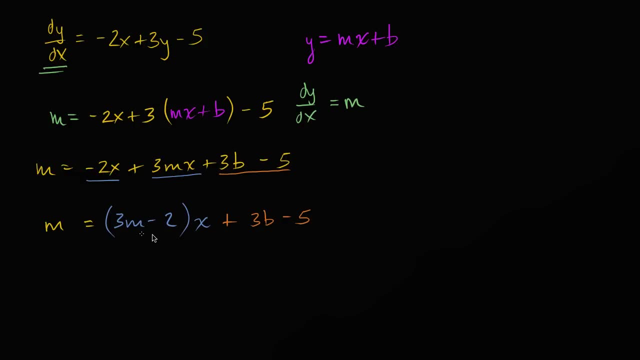 So notice, over here I have some coefficient times: x on the right hand side, but on the left hand side I have no x's. So somehow this thing must disappear. This is a constant, so it's completely reasonable. it's completely reasonable that this constant 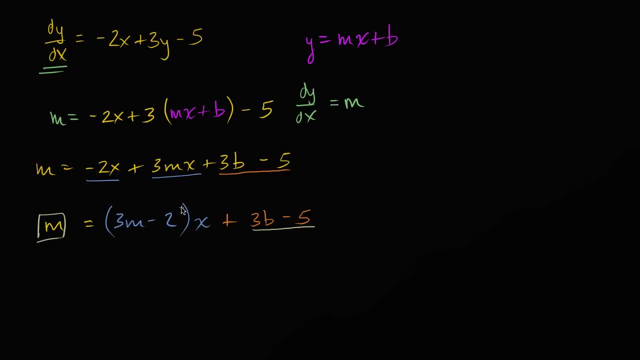 could be equal to m, but the only way that I get these x's to disappear- so all I'm left with is an m- is if this thing is equal to zero. Let me say that again because I think it might maybe be a little bit. 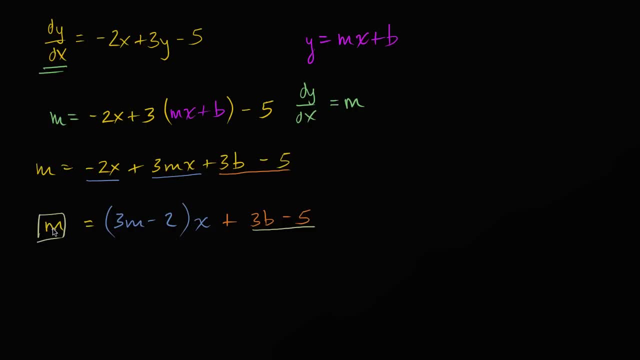 a little bit counterintuitive what I'm about to do. We're saying that m some constant value is equal to some coefficient times x plus some other constant value. Well, in order for a constant value to be equal to a coefficient times x, 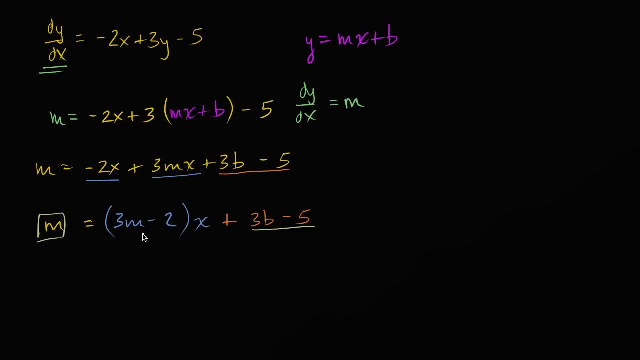 plus some other constant value, the coefficient on x must be equal to zero. Another way to think about it is this should be: you could rewrite the left hand side here as zero x plus m, And so you see, you kind of match the coefficients. 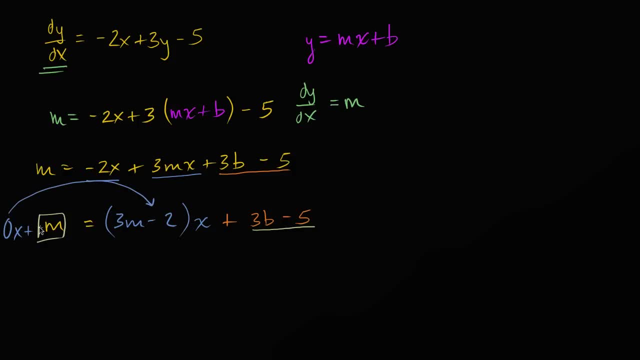 So zero must be equal to three m minus two, and m is equal to three b. m is equal to three b minus five, m is equal to three b minus five. So let's use that knowledge, that information, to solve for m and b. 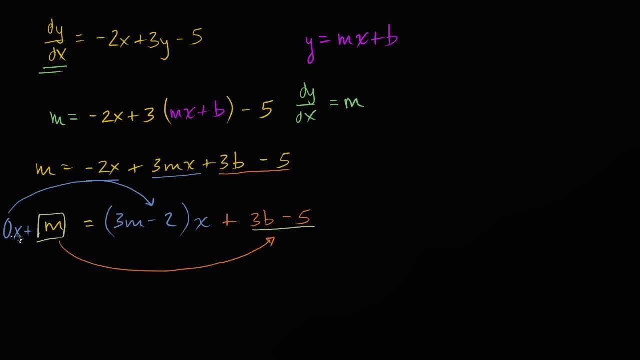 So we could use this first one. so three m minus two must be equal to zero. So let's write that three m minus two is equal to zero, or three m is equal to two, or m is equal to two thirds. so we figured out what m is. 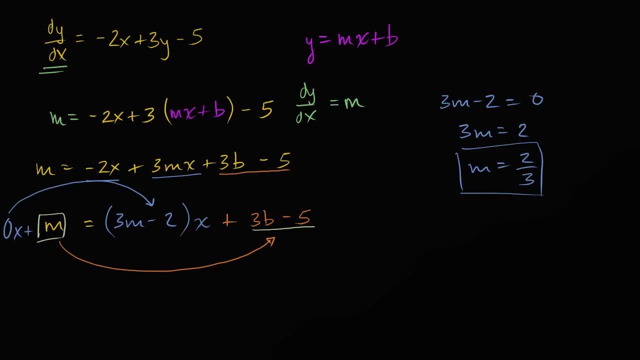 And then we could use that information, because we know that. we know that m is equal to is equal to three b minus five. m is two thirds. so we get: two thirds is equal to three b minus five. We could add five to both sides. 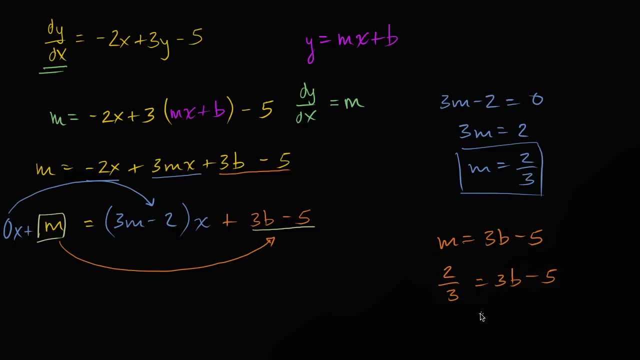 which is the same thing as adding 15 thirds to both sides. Is that? did I do that right? Yeah, it's, adding five to both sides is the same thing as adding 15 thirds to both sides, so let's do that. 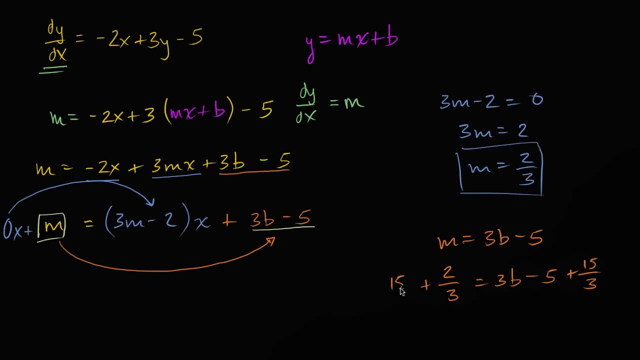 15 over three plus 15 over three, These cancel out. that's just five. right over there on the left-hand side, We have 17 over three is equal to three b, or if you divide both sides by three, you get b is equal to 17,. 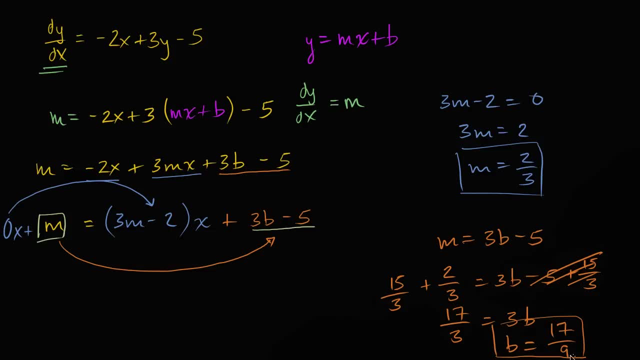 b is equal to 17 over nine. And we're done. We just found a particular solution for this differential equation. The solution is: y is equal to two thirds x plus 17 over nine. And I encourage you after watching this video. 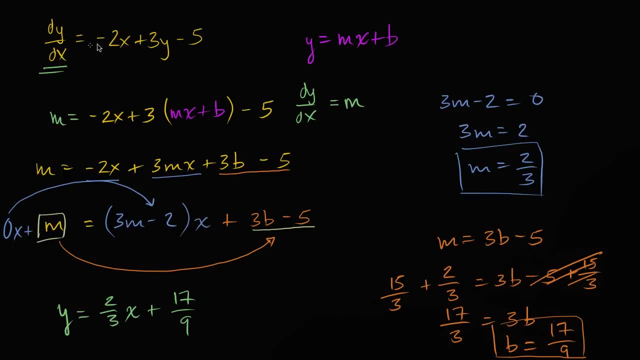 to verify that this particular solution indeed does satisfy this differential equation. for all x's, For all x's. Thank you.